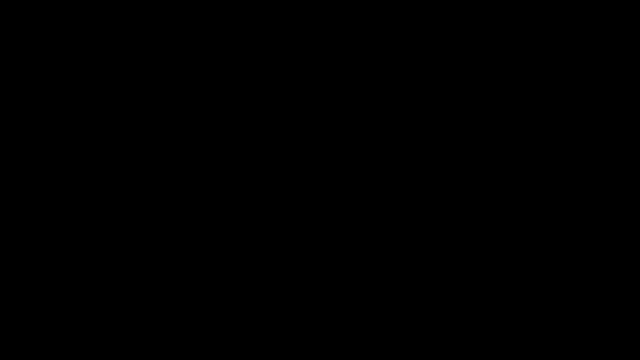 In this video we're going to talk about the ratio test, And so here's the basic idea behind it. Let's say, if we take the limit, as n goes to infinity, of the absolute value of a sub n plus 1 divided by a sub n, 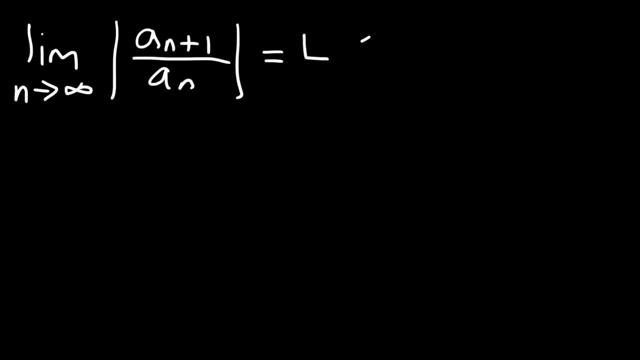 And let's say we get some limit l and that limit is less than 1. Then the series is going to be absolutely convergent. Now let's say: if we take the same limit, but this time I'm going to write it differently. 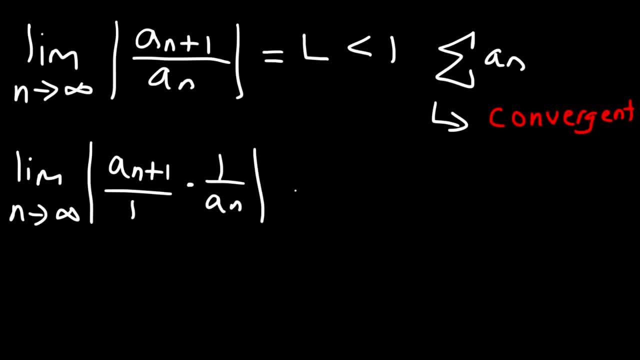 Because you can write it this way if you want to. Now, let's say it's greater than 1, or if the limit goes to infinity, then the series is going to be divergent. Now, the third way to write it is to take the limit as n. 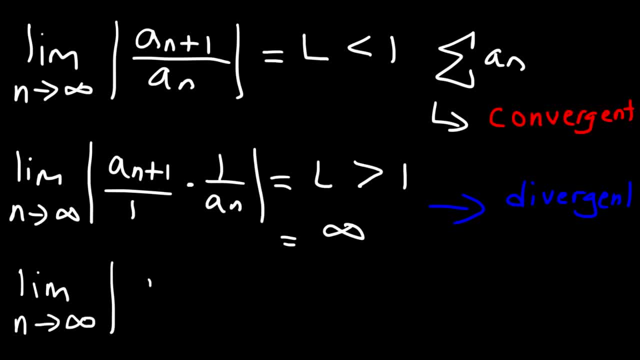 The third scenario has to do with the limit being equal to 1.. If it's equal to 1, then the series we can say is inconclusive. You can't make no conclusion about it using a ratio test. You may have to use some other tests. 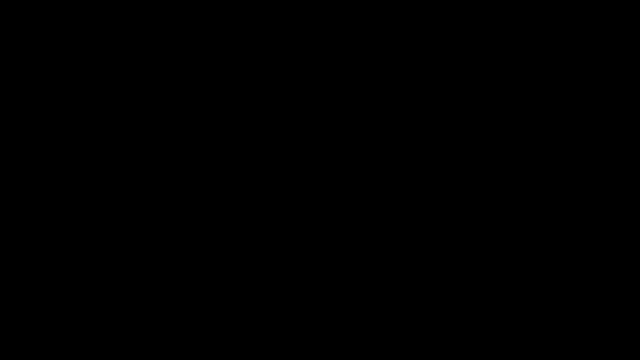 So that's the basic idea behind a ratio test. And now let's work on some examples. So consider the series of 3 to the n over n factorial, So go ahead and use the ratio test to determine if the series is going to converge or if it's going to diverge or if it's going to be inconclusive. 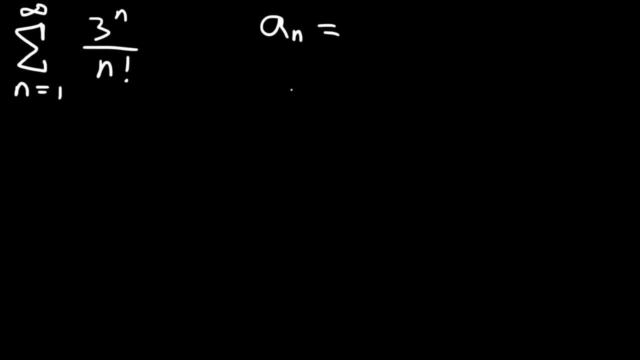 So first let's define a sub n and a sub n plus 1.. So a sub n is going to be 3 to the n over n factorial, And a sub n plus 1 is going to be 3 to the n plus 1 divided by n plus 1 factorial. 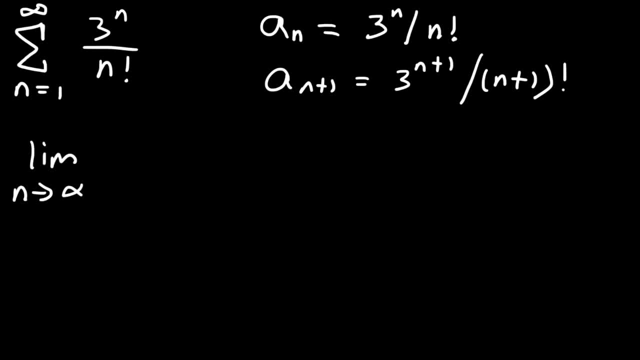 So now let's take the limit as n goes to infinity of a sub n plus 1 times 1 over a sub n, So this is going to be 3 to the n. So let's take the limit as n goes to infinity of a sub n plus 1 times 1 over a sub n. 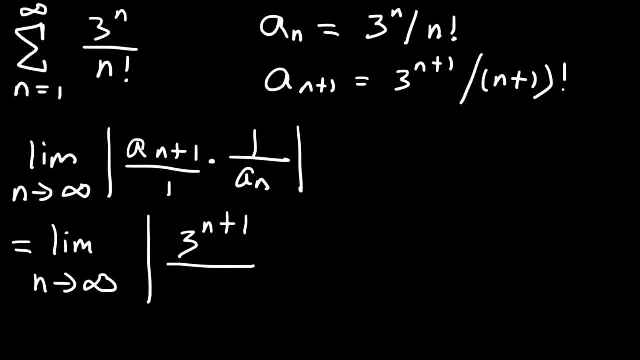 plus 1 divided by n plus 1 factorial. Now, if this is a to the n, then a sub n is going to be the reciprocal of that. It's going to be n factorial divided by 3 to the n. Now 3 to the n plus 1.. How can we simplify that 3 to the n plus 1,? 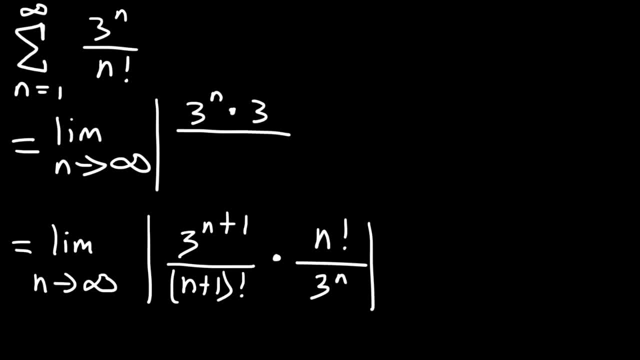 that's 3 to the n times 3.. n plus 1- factorial: you can write that as n plus 1 times n factorial, And I have a video on factorials and how to simplify it if you want to look it up on YouTube. 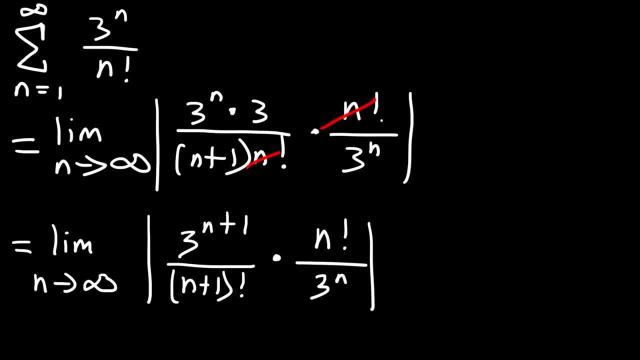 So you want to simplify it in such a way that you can cancel a few things. Let me use a different color for that. So what we have left over is the limit, as n goes to infinity, of 3 over n plus 1.. So when n becomes large, 3 over n plus 1 is going to go to 0.. 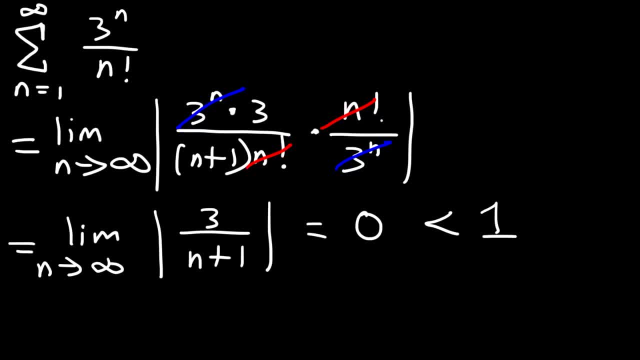 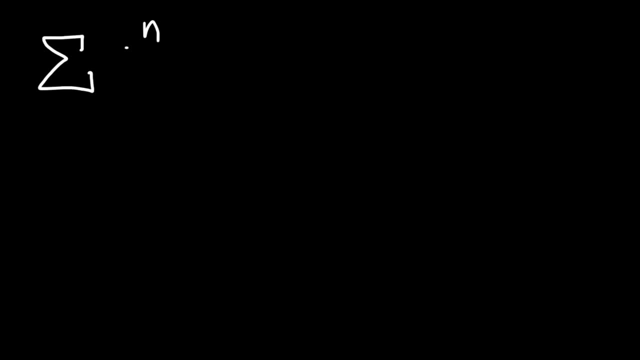 And 0 is less than 1.. So therefore, we could say that the original series converges absolutely, And so that's the answer. Now let's go ahead and work on some more examples. So let's say, if we have n over 4 to the n, 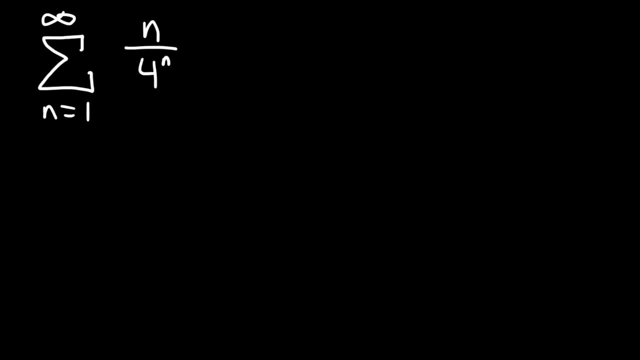 Go ahead and use the ratio of n to the n, Go ahead and use the ratio of n to the n, And then we're going to use the ratio test to determine if this series is going to converge or if it's going to diverge. 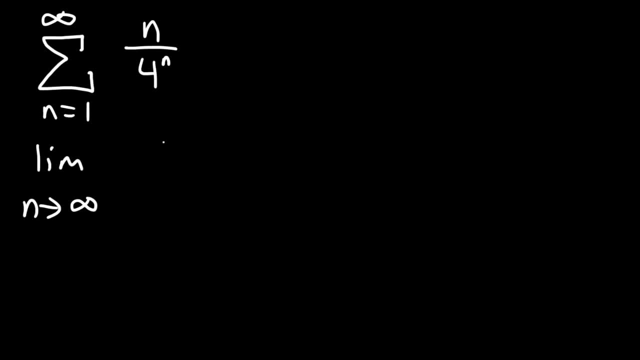 So let's start with the limit, as n goes to infinity, of a sub n plus 1 times 1 over a sub n. So that's going to be the limit as n approaches infinity, And then a sub n plus 1, that's going to be this expression, but everywhere we see an n. 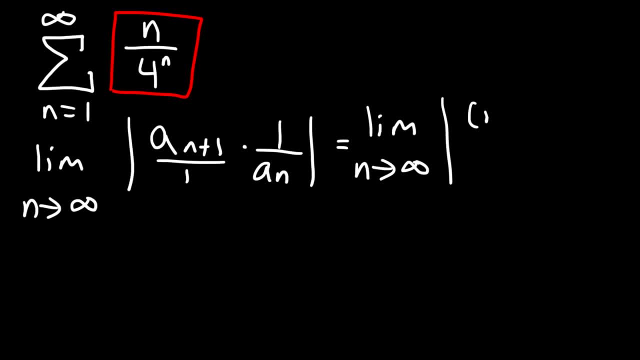 let's replace it with n plus 1.. So we have an n on top, so we're just going to put n plus 1.. And then, instead of 4 to the n, it's going to be 4 to the n plus 1.. 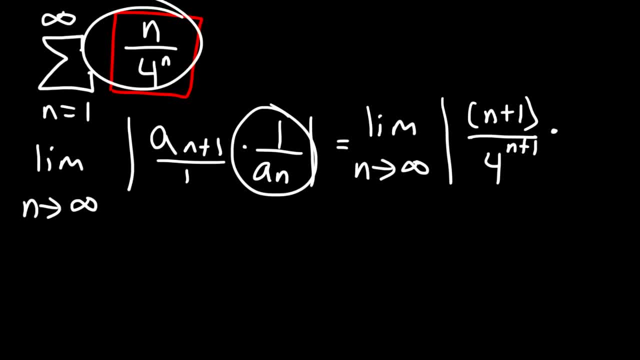 And then we're going to multiply it by the reciprocal of this expression. So let's flip the fraction and it's going to be just 4 to the n divided by n. Now I'm going to rearrange the terms, So I'm going to move this. 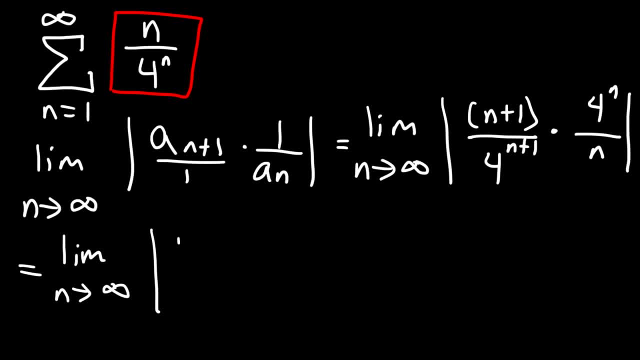 I'm going to move this over here. So I'm going to have n plus 1 divided by n times 4 to the n, And then 4 to the n plus 1, I can write that as 4 to the n times 4.. 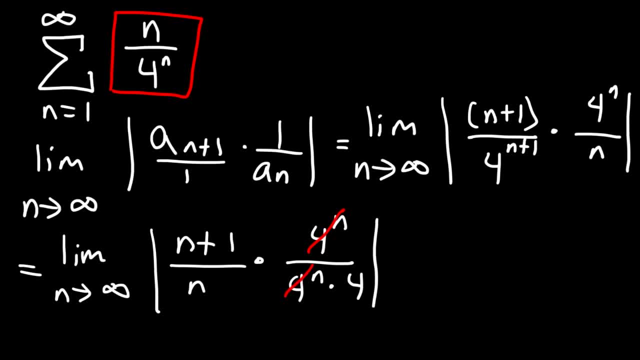 And so these two can be cancelled, And so I'm left with 4, I mean not 4, but that's going to be 1 over 4 if I move that to the front, since it's on the bottom, So it's 1. fourth, the limit, as n goes to infinity. 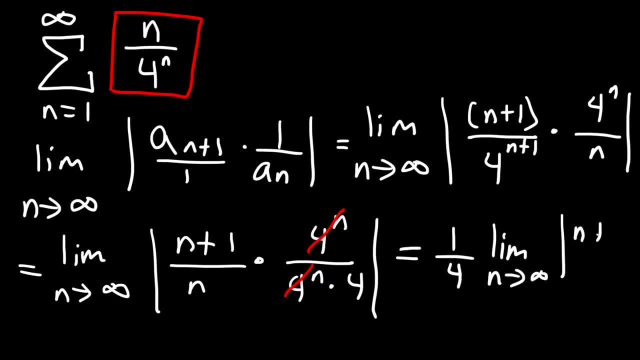 And then I have n plus 1 divided by n. So when n becomes very large, what's going to happen to n plus 1 over n? Well, if you're not sure, we can do some more work to simplify it. So what I'm going to do is, on the inside, I'm going to multiply the top and bottom by 1 over n. 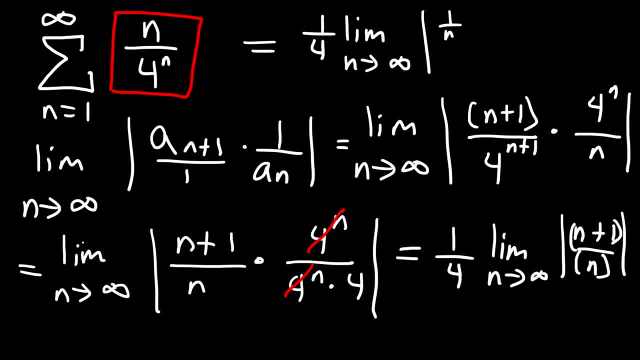 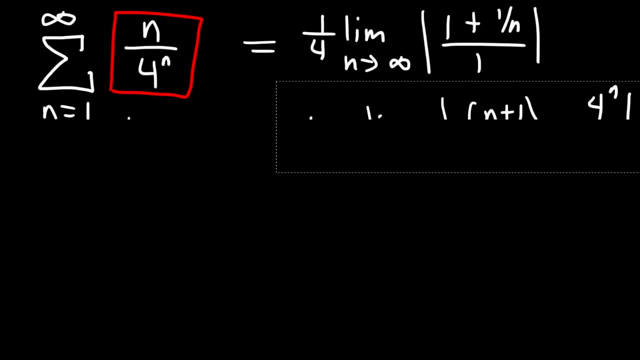 So it's going to be 1 over n. So it's going to be 1 over n. Actually, this is going to be 1 plus 1 over n, divided by 1.. Now, as n goes to infinity, 1 over n approaches 0.. 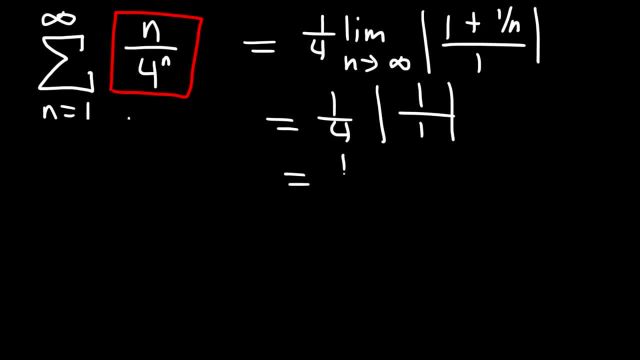 So this becomes 1 over 1, so it's just 1 fourth times 1, which is 1 over 4.. And 1 over 4 is less than 1.. So we can say that the original series converges. 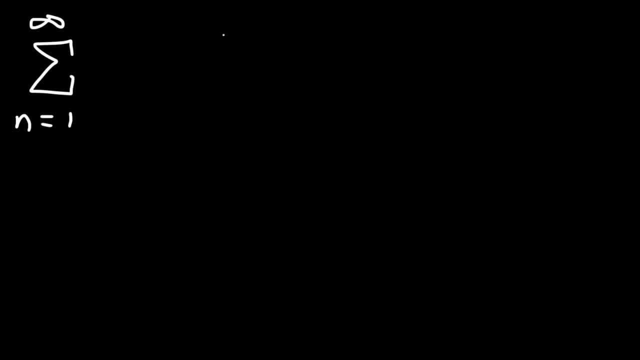 Now let's try another example. So let's say: this time it's 3 to the n plus 2 times n squared divided by 4 to the n. So let's use the ratio test to see what's going to happen. So let's start with the limit, as n goes to infinity. 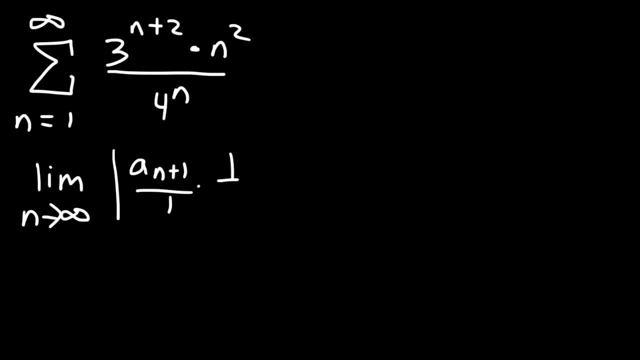 Of a sub n plus 1 times 1 over a sub n. I'm going to need more space, So a sub n plus 1.. Everywhere we see an n, replace it with n plus 1.. So we're going to have 3 times n plus 1 plus 2.. 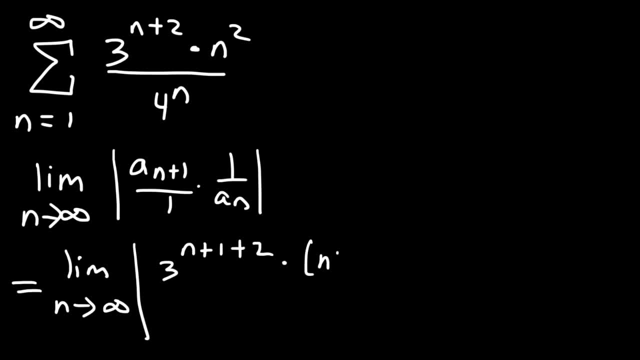 And then, instead of n squared, it's going to be n plus 1 squared divided by: Instead of 4 to the n, it's going to be 4 to the n plus 1.. Now let's multiply it by the reciprocal of that fraction. 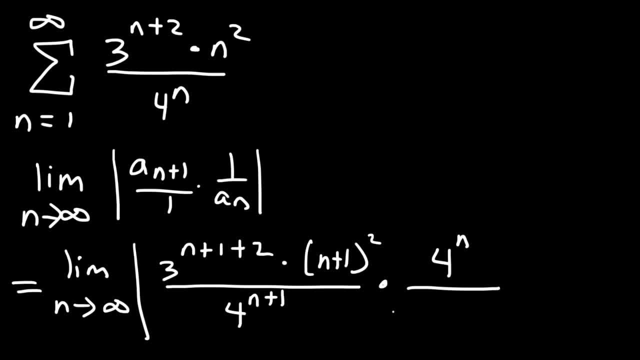 So that's going to be 4 to the n divided by 3 to the n plus 2 times n squared. Okay, So let's simplify Now. what do you think I should do with this term? Notice that I have a 3 to the n plus 2 there. 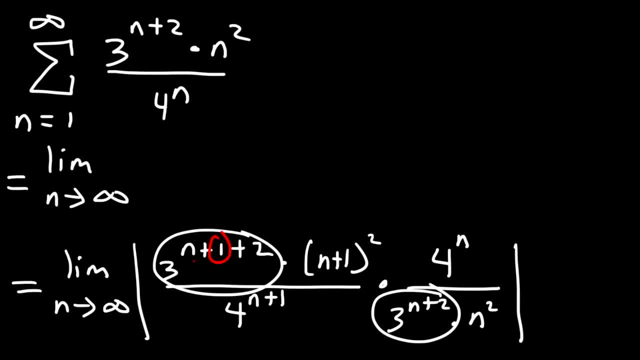 So what I want to do is I want to separate the 1 from the n plus 2.. So 3 to the n plus 1 plus 2, I'm going to write it as 3 to the n plus 2 times 3 to the 1.. 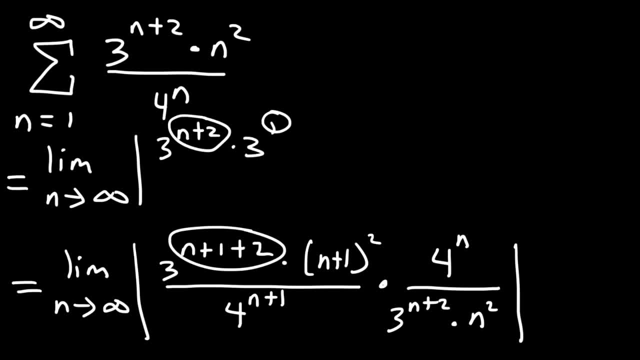 Because n plus 2 plus 1 is the same as that expression. Now 4 to the n plus 1, I'm going to write it as 4 to the n times 4 to the first power, n plus 1 squared. I'm just going to leave it the way it is. 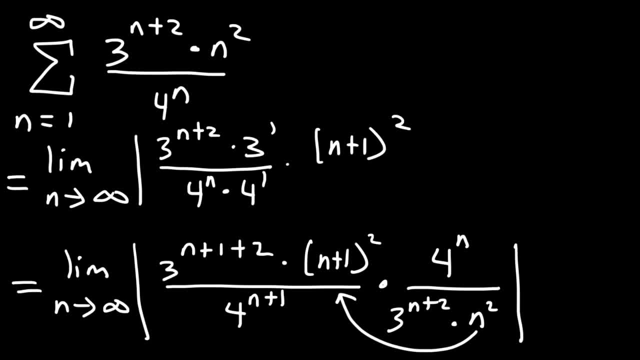 But I'm going to take this part and move it right under n plus 1 squared, And then everything else. I'm just going to leave it The way it is. Now. we could cancel 4 to the n And we can cancel 3 to the n plus 2.. 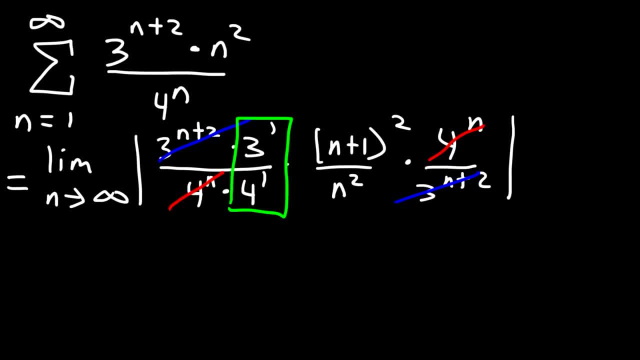 So now the constant 3 over 4, let's take it outside of the absolute value expression. So if we move it to the front, we're going to have 3 over 4 times the limit, As n goes to infinity, of n plus 1 squared over n squared. 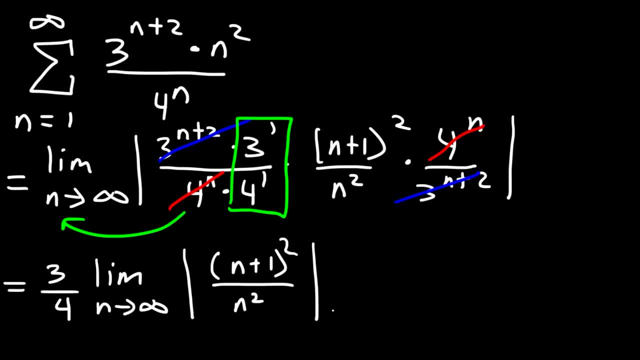 Now, what do you think we need to do at this point? Well, let's go ahead and expand n plus 1 squared. So if you FOIL n plus 1 times n plus 1, you should get n squared plus 2n plus 1.. 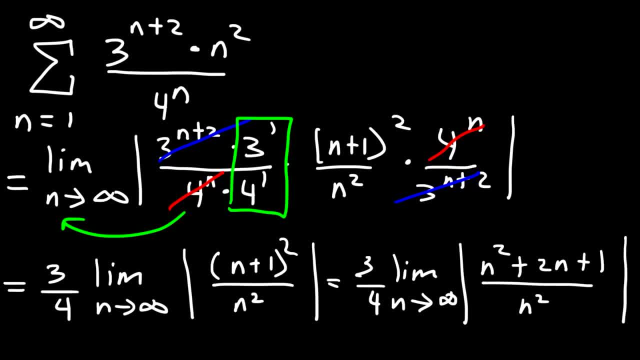 So if you FOIL n plus 1 times n plus 1, you should get n squared plus 2n plus 1.. So what I'm going to do now is I'm going to multiply the top and the bottom by 1 over n squared. 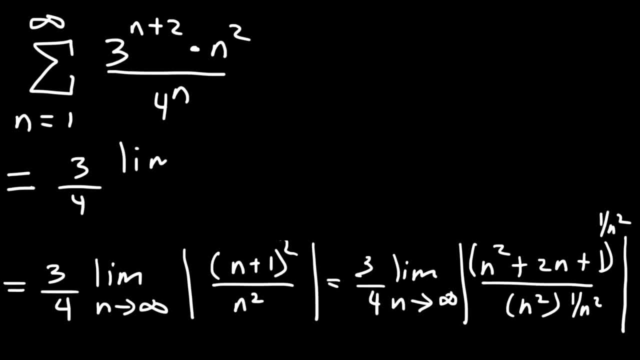 And so now I'm going to have n squared times 1 over n squared, that's just going to be 1.. And then 2n times 1 over n squared, that's going to be 2 times 1 over n. 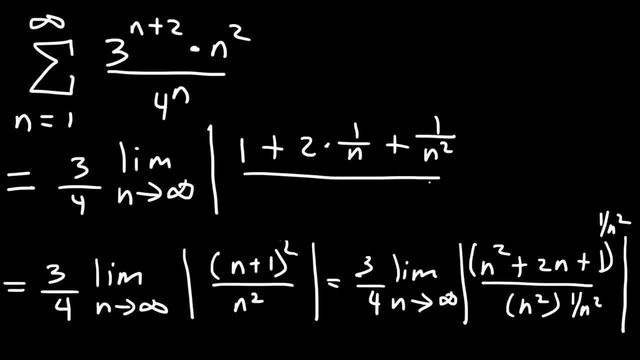 And then we're going to have plus 1 over n, squared, divided by 1.. So we really don't need to write divided by 1 at that point. We could just leave it like this: So when n becomes very large, what's going to happen? 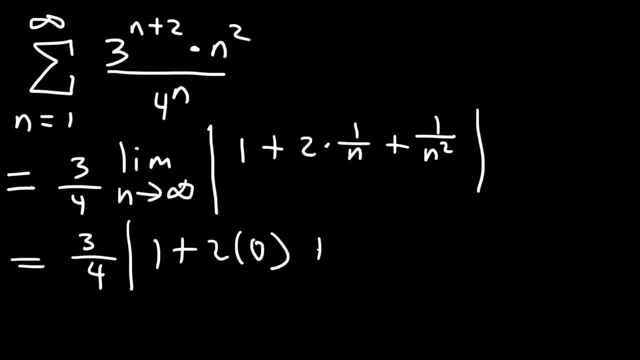 1 over n will become 0. And 1 over n squared will also approach 0. So we're just going to have 3 over 4 times 1. And so the limit is equal to 3 over 4.. And 3 over 4 is less than 1,. 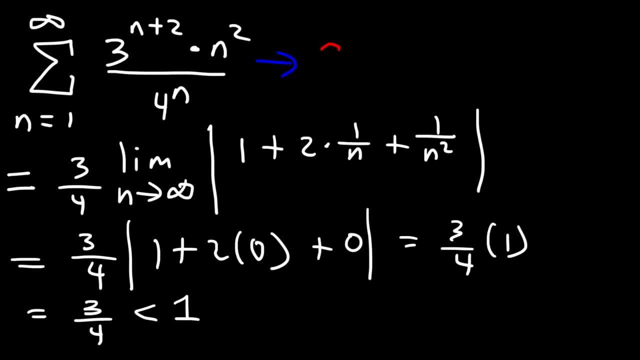 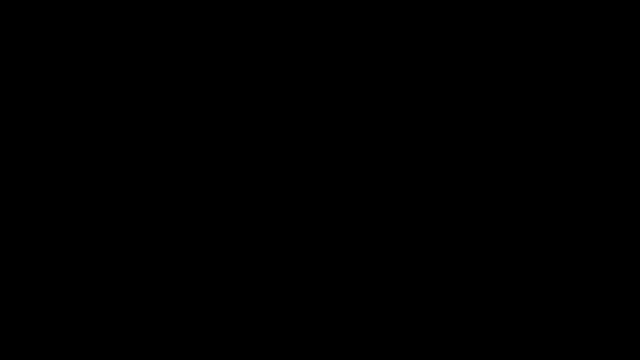 which means that the original series is absolutely convergent. Now let's move on to our next step, To our next example problem. So what about n to the n over n factorial? Will it converge or will it diverge? Go ahead and try that. 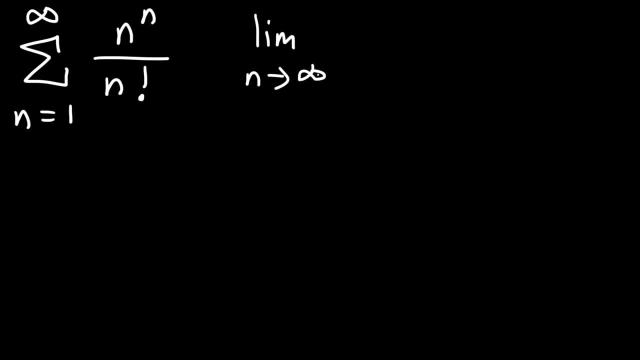 So let's start with the limit, as n goes to infinity, And then a sub, n plus 1.. That's going to be n plus 1 raised to the n plus 1 divided by n plus 1.. And then times. let's multiply it by the reciprocal of this. 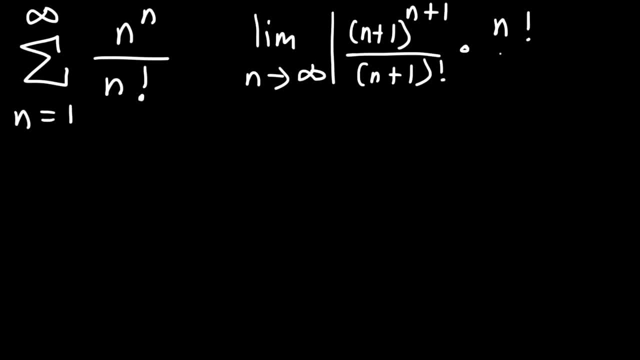 or 1 over a sub n. So that's going to be n factorial divided by n to the n. So how can we simplify this expression? What do we need to do? So the first thing I would try to do is make sure that these exponents are the same. 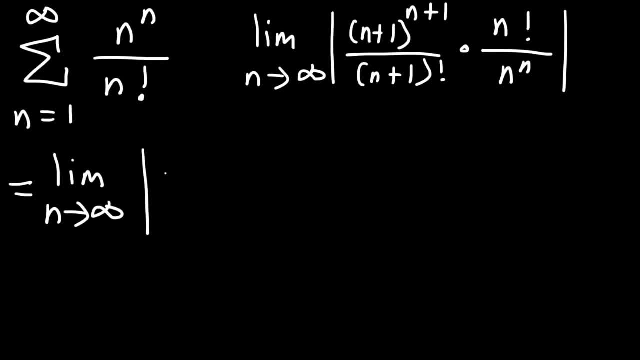 So n plus 1 to the n plus 1, we can write that as: n plus 1 to the n times n plus 1 to the first power, Now n plus 1 factorial, that's n plus 1 times n factorial. 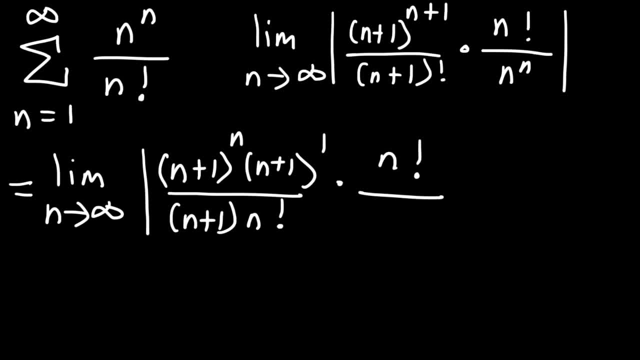 And so we can easily cancel out the n factorial expression. So these will cancel. In addition, n plus 1 will also cancel as well. So what we have left over is n plus 1 to the n, divided by n to the n. 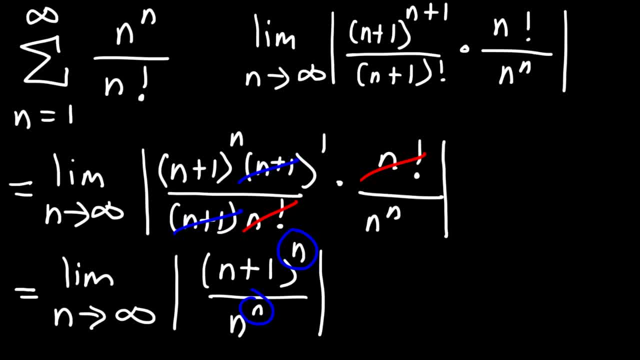 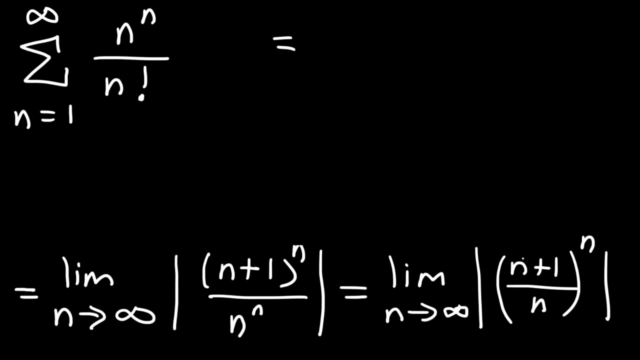 Now, because the exponents are the same, we can write it like this: We can say it's n plus 1 over n raised to the n. So I'm going to continue the work up here Now. n divided by n. 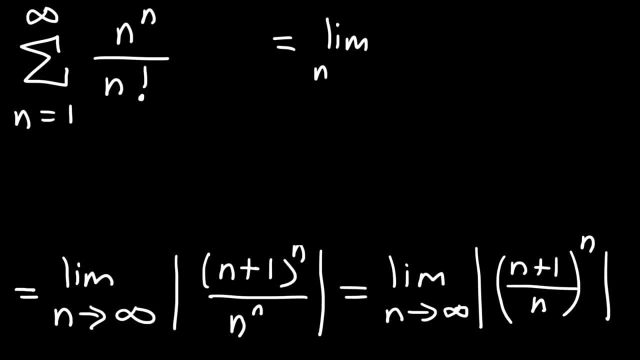 that's 1.. And then we have 1 divided by n. So I'm just going to write that as 1 over n to the n, 1 over n, And all of this is raised to the nth power. So what is the limit? 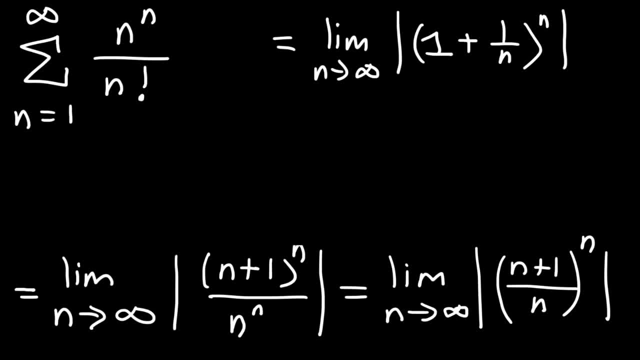 as n goes to infinity of 1 plus 1 over n raised to the n. Well, if you're not sure, here's what you can do: We're going to set the limit equal to y. Let's not worry about the absolute value symbol. 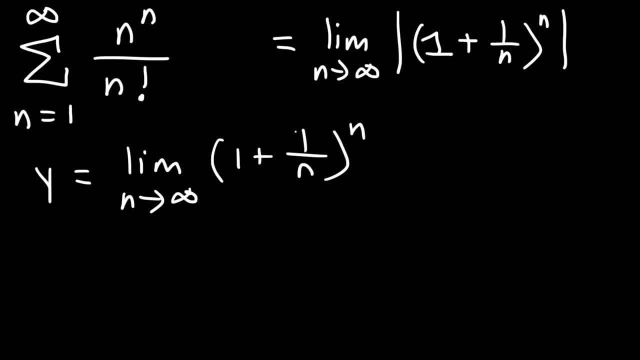 because n is positive, So this whole thing is going to be positive. Now what we need to do is take the natural log of both sides, And so if we do that, we can now take the exponent and move it to the front. 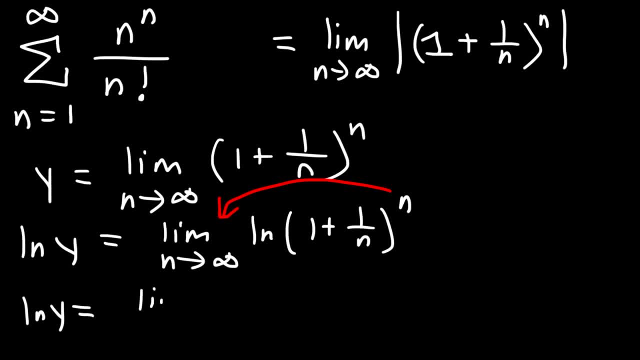 So we're going to have: the natural log of y is equal to the limit, as n goes to infinity, of n times the natural log of 1 plus 1 over n. Now we need to use L'Hopital's rule, But we need to put it in a form. 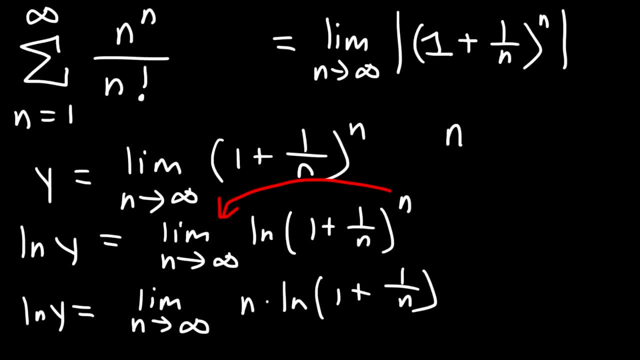 that works for L'Hopital's rule. So it's important to understand that n is the same as 1 over 1 over n. So now we have the natural log of y is equal to the limit, as n goes to infinity, And then it's going to be the natural log. 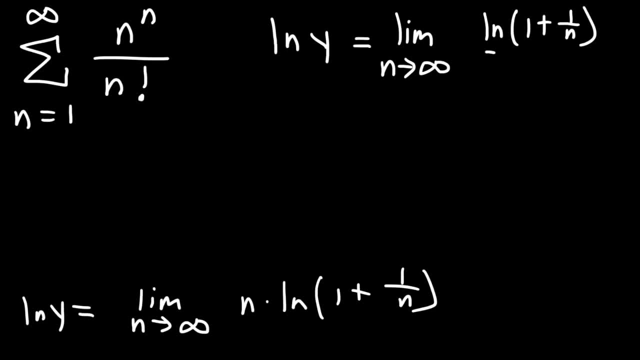 of 1 plus 1, divided by n over 1 over n. So now let's take the derivative of the top and the bottom. So what is the derivative of Ln? 1 plus 1 over n? If you recall the derivative of Lnu, 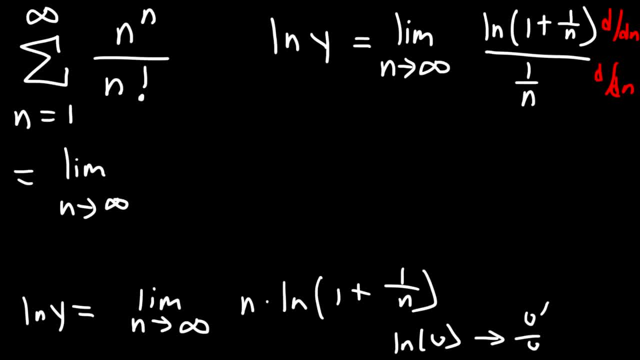 is u prime over u. So u is this expression, The derivative of u is u prime over u. The derivative of that is going to be the derivative of 1 over n, which is just negative 1 over n squared. And then we need to divide it. 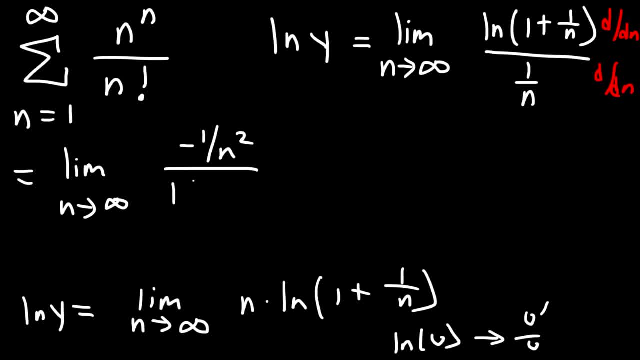 by the original expression that was on the inside. So that's 1 plus 1 over n, And then the derivative of this, 1 over n. that's going to be negative 1 over n, squared using the power rule. So this is what we now have. 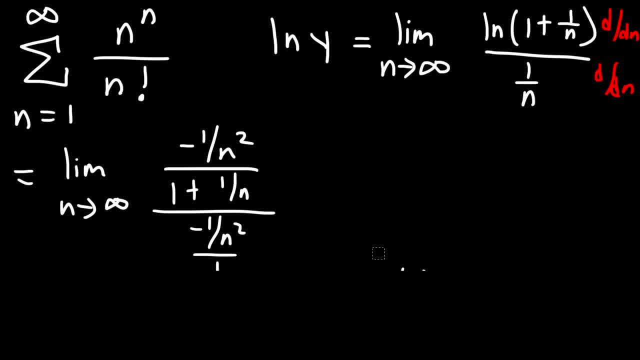 Now let's multiply the top and the bottom by negative n squared. So if we do that, this is what we're going to get. So this fraction times negative n squared, the negative 1 over n squared and the negative n squared, will cancel. 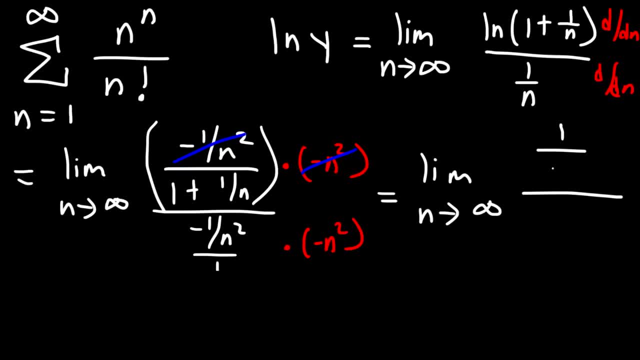 So we're going to get a 1 on top. So we're going to get a 1 on top And then on the bottom, it's just going to be 1 plus 1 over n. Now, once we multiply these two, 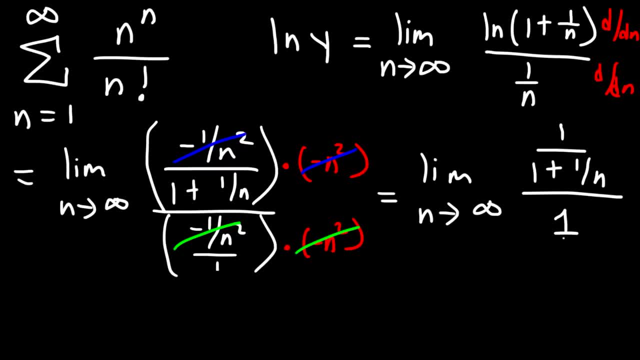 they will cancel completely, And so we're just going to get a 1 on the bottom So we can write the whole thing as the limit, as n goes to infinity: 1 over 1 plus 1 over n, Because when you divide something by 1,. 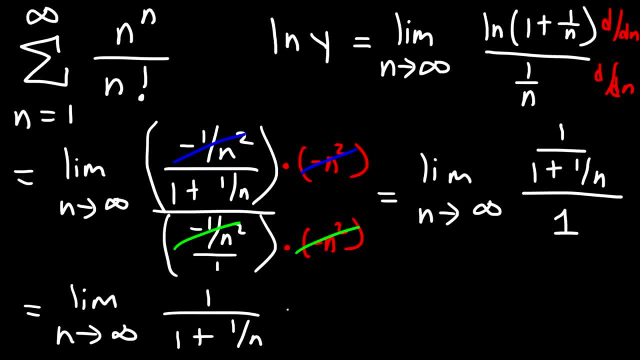 it really doesn't matter. Now, keep in mind: all of this is equal to the natural log of y. Now, as n goes to infinity, 1 over n approaches 0. And so this is equal to 1.. And 1 is equal to ln, y. 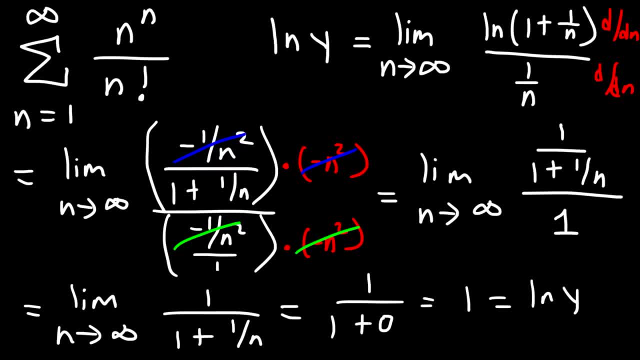 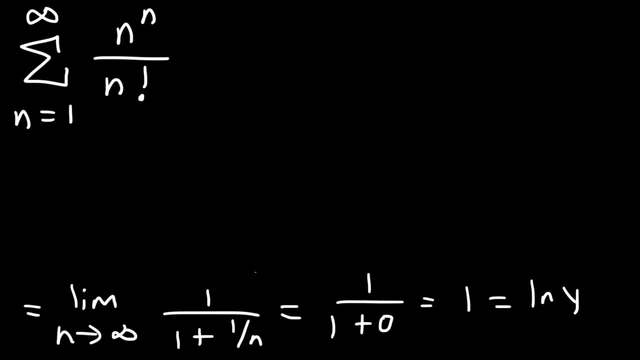 But recall that the original limit that we're trying to find is equal to y, not ln y. So our goal is to solve for y. So if ln y is equal to 1, what is the value of y? Now, keep in mind, the base of a natural log expression is e. 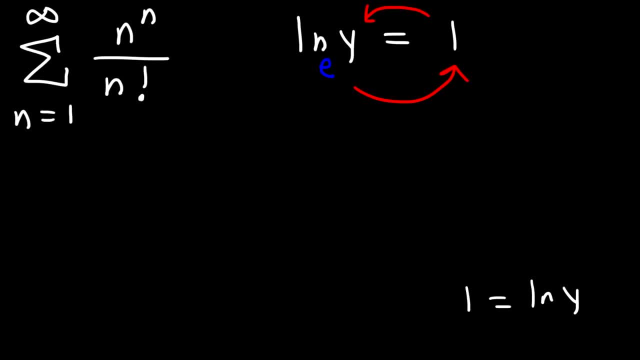 So e raised to the 1, power is equal to y, So y is equal to e And if you recall y, we set it equal to the limit, as n goes to infinity, of 1 plus 1 over n raised to the n. 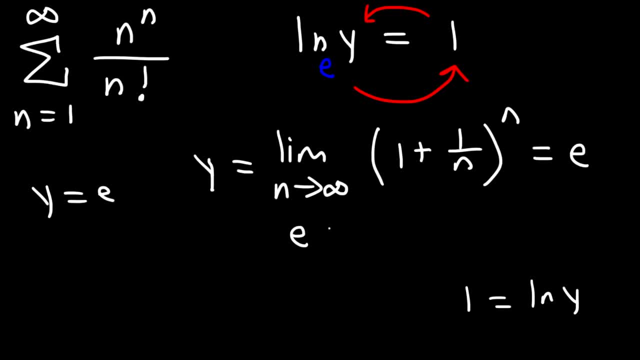 And so that is equal to e. Now, e is greater than 1. And because of that this series diverges. And that's the answer for this problem. Let's work on this one. So let's say, if we have 2 raised to the 4, n plus 1 divided, 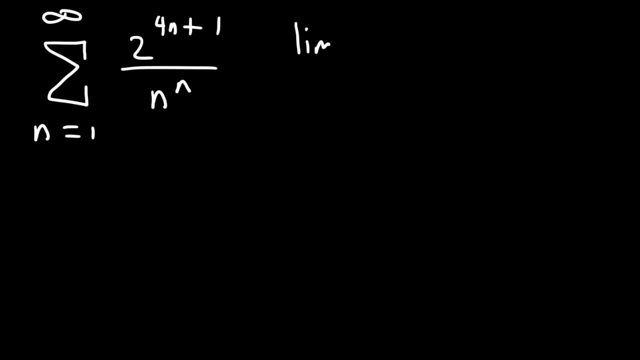 by n to the n. So let's take the limit, as n goes to infinity, And then it's going to be sub n plus 1.. So everywhere we see an n, we're going to replace it with n plus 1.. And so n to 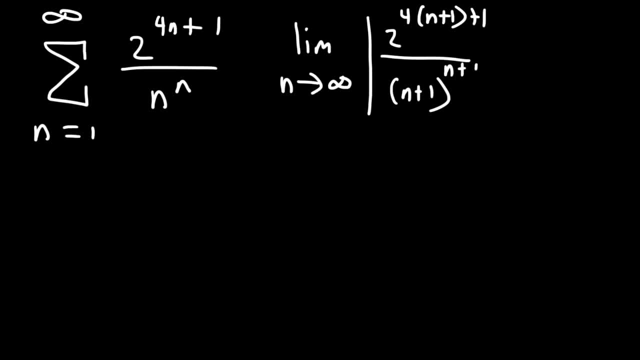 the n, that's going to be n plus 1 raised to the n plus 1.. And then we're going to multiply it by the reciprocal of a sub n. Now let's see what we can do to simplify that expression. So if we distribute the 4, this would be 2 to the 4n plus 4 plus 1.. But I want to separate 4n. 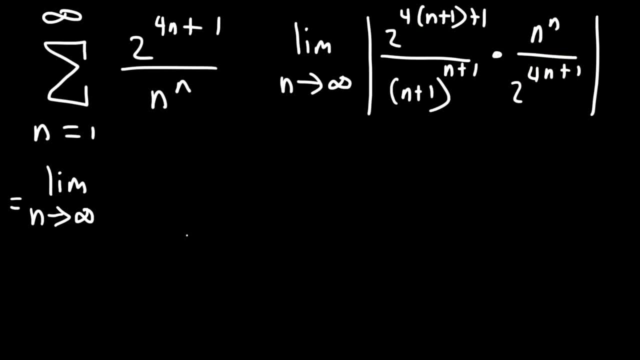 plus 1 from the 4.. Right now I'm just going to write it the way it is, So it's 2 to the 4n plus 4 plus 1.. But what I want to do is switch these two, So I'm going to write it as 1 plus 4 instead. 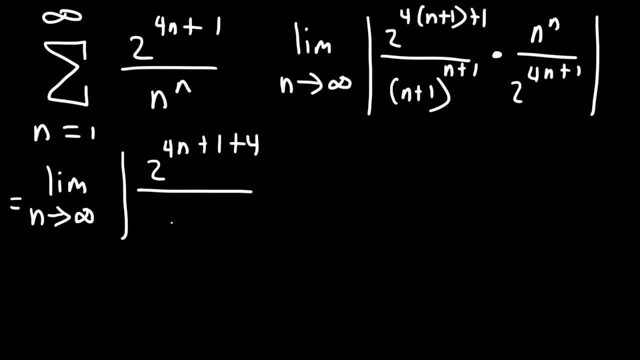 Now n plus 1 raised to the n plus 1.. That's going to be n plus 1 raised to the n times n plus 1 raised to the 1.. So now 2 to the 4n plus 1 plus 4.. Let's separate the 4n plus 1 from the 4.. 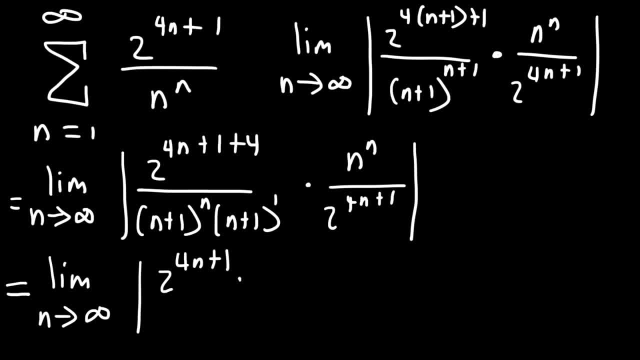 So we're going to have this times 2 to the 4.. And this I'm going to rewrite it right below it. So divide it by 2 to the 4n plus 1.. Now these two. I want to write it together because 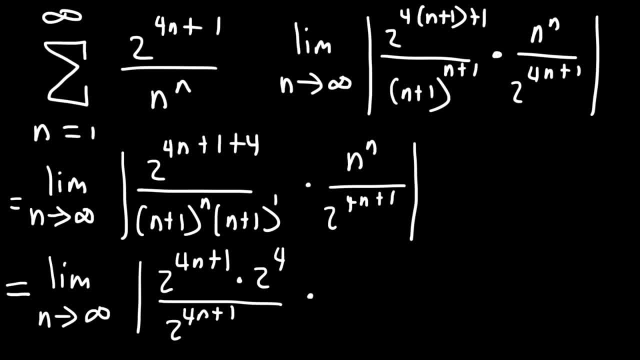 they share the same exponent. So I'm going to have times n to the n over n plus 1 raised to the n power, And then this- I'm just going to leave it by itself for now. So 1 over n plus 1.. So these will cancel. And 2 to the 4th power is 16, which I can move to the 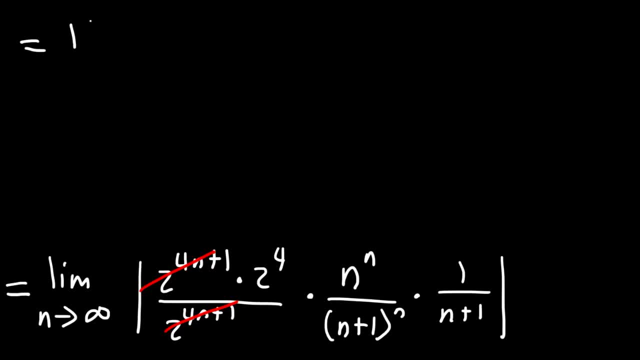 front. So now I have 16 times the limit, as n goes to infinity. And then it's going to be n divided by n plus 1, raised to the n power times, 1 over n plus 1.. Now let's separate this into two parts. 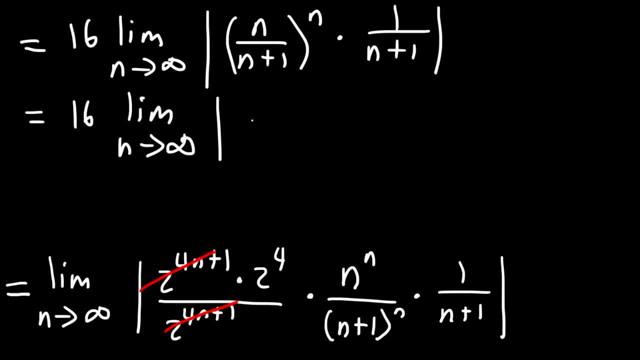 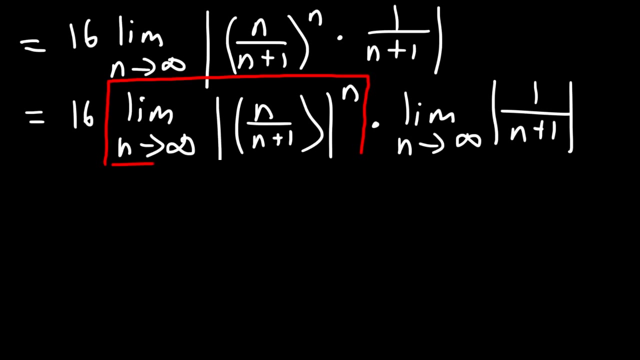 So this is going to be the first part, And then this is going to be the second part. So this is going to be the first part, And then this is going to be the second part. Now let's analyze this limit. as n becomes very large, What does this expression turn into? 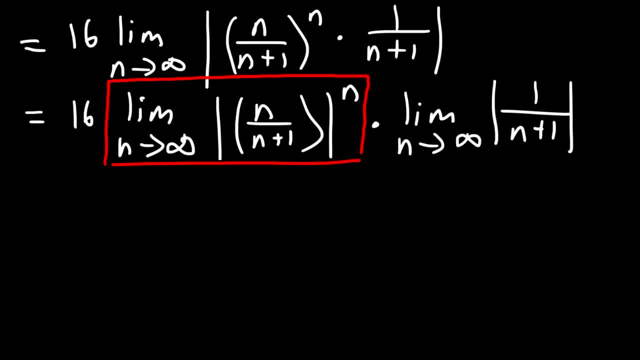 Well, if you plug in, let's say, a thousand for n, you're going to have a thousand divided by a thousand and one raised to a thousand. So now let's say I have a total of one. COME stock of N to. raise to a thousand, And then this expression gets Seka the 10th to the 10th power. So now let's know the units here, And let's remember that this is the new limit, and I'm taking the N to N plus N. 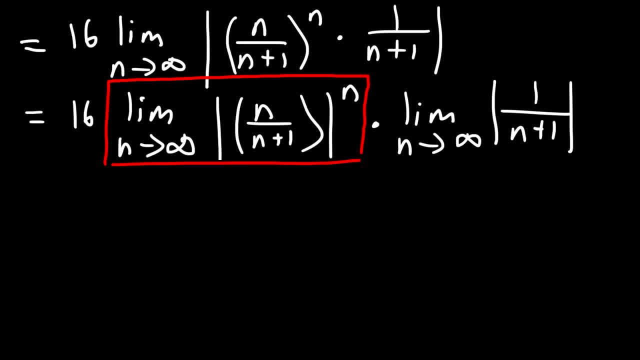 And so you should get 0.36806.. And it turns out that it converges to 1 over E. 1 over E is like 0.367879.. If you follow the same process that we did before, if, let's say, you set it equal to Y. 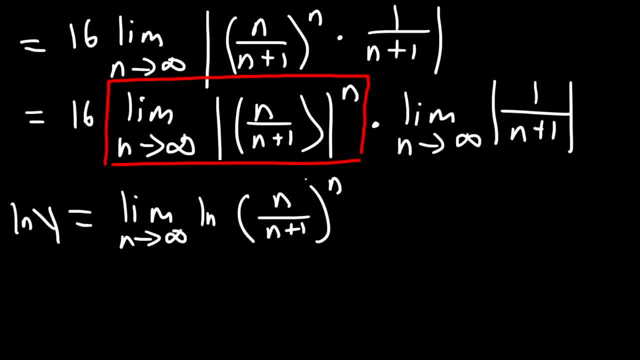 and then if you take the natural log of both sides and then bringing this to the front and then putting it in a form where you can do L'Hopital's Rule, So this is going to be 1 over N- now You'll find that this will converge to 1 over E. When you solve for Y, you should get 1. 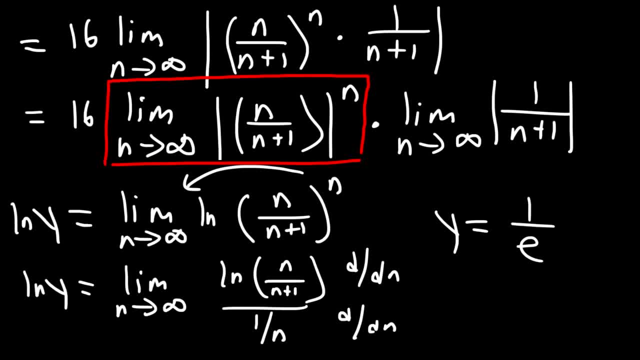 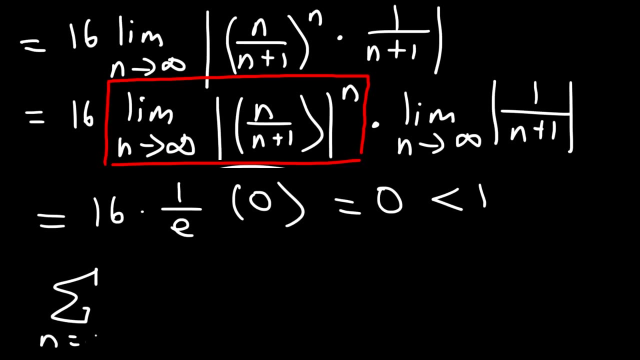 over E. In either case, 1 over E is a constant, So we're going to have 16 times 1 over E and then, when N becomes large, 1 over N plus 1 will approach 0. So the whole thing is 0,, which is less than 1,, which means that the original series it. 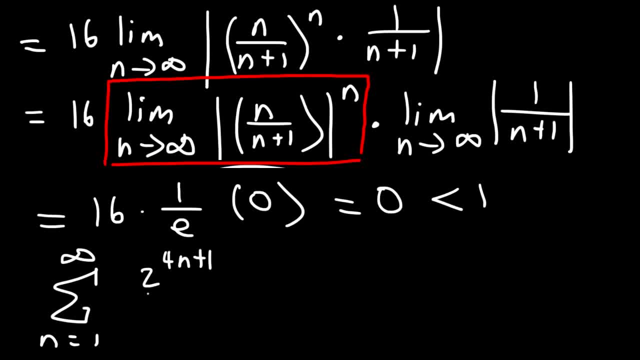 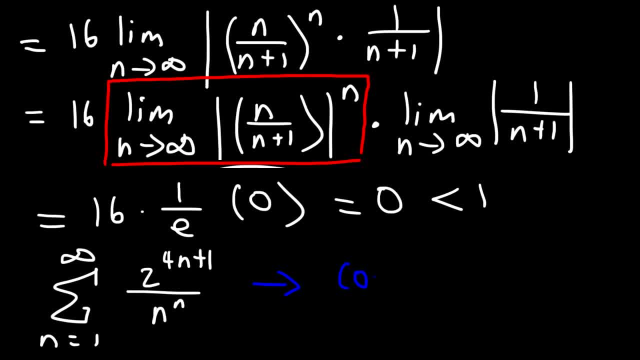 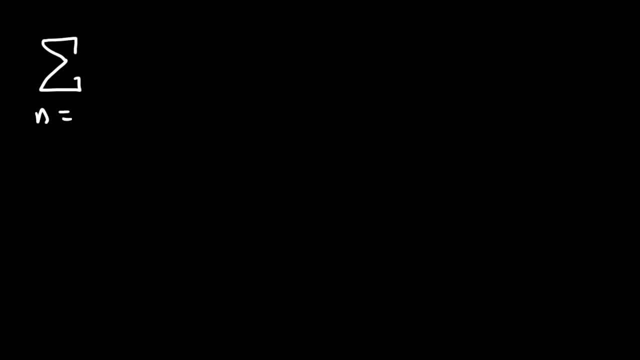 the 4N plus 1 over N to the 5N plus 1 over N, this series will converge. Consider this problem. Let's say we have negative 1 to the N plus 1 times N plus 2 divided by the square root. 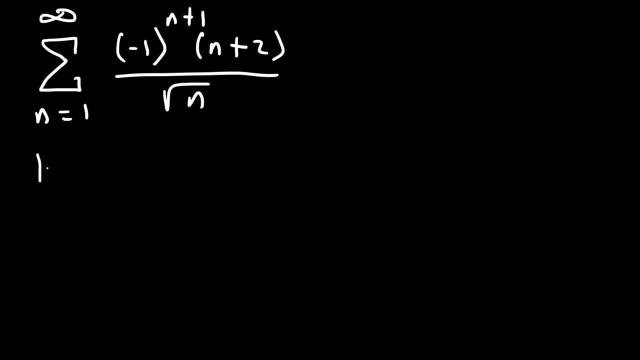 of N. Go ahead and try that. So using a ratio test. we're going to have this Now, since we're going to take the absolute value, we're going to have this value of the ratio of a sub n plus 1 to a sub n, the negative 1 raised to the n plus 1 of this. 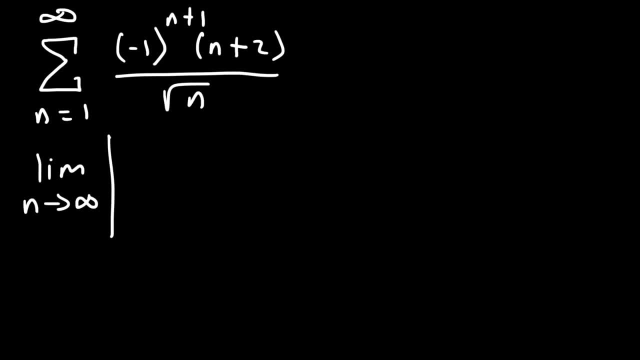 alternate series is going to disappear. it's not going to be important. so, therefore, a sub n is now just n plus 2 divided by the square root of n, and a sub n plus 1, that's going to be n plus 3 divided by the square root of n plus 1. so we're going to start with this one first. 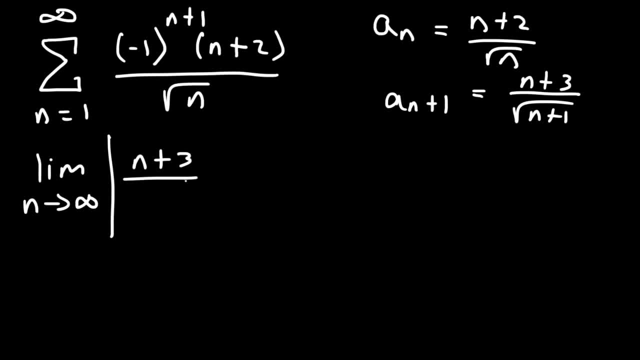 and then we're going to multiply it by the reciprocal of a sub n. now let's rewrite the expression like this: so i'm just going to reorganize it. i'm going to put the n plus 2 underneath the n plus 3, and then the square root of n plus 1. i'm going to put it under the square root of n. 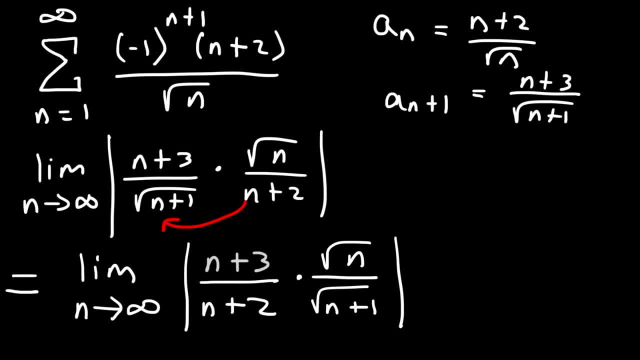 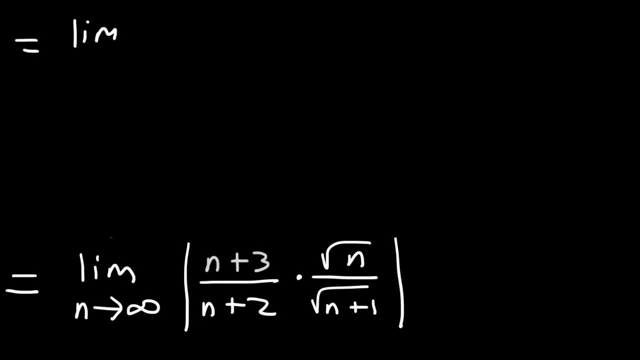 and then let's separate it into two limits. so the first limit is going to look like this: n plus 3 over n plus 2 times the second limit, which we can write that all within a single square root symbol. so that's just going to be n. 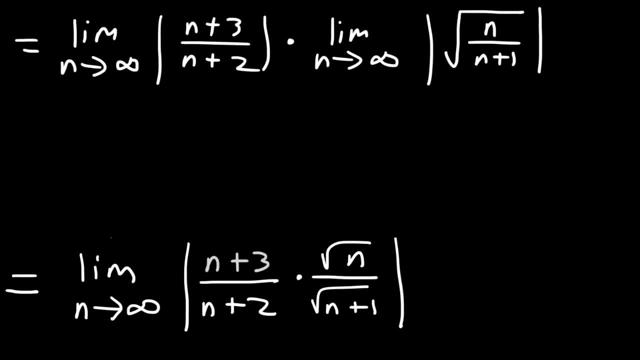 divided by n plus 1. now we're going to multiply n plus 3 and n plus 2 by 1 over n. so if we do that we're going to have the limit as n goes to infinity, and then it's just going to be 1 plus 3 times 1 over n. 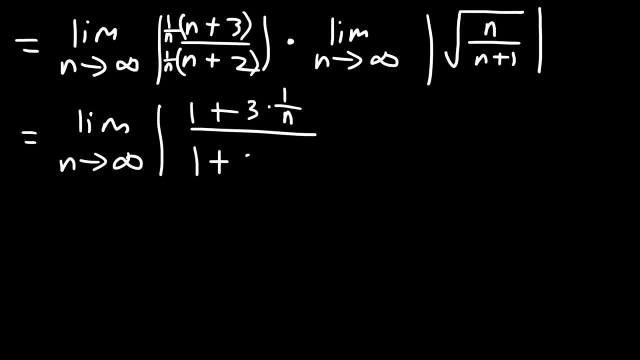 and then divided by 1 plus 2 times 1 over n. now for the second one. we're going to do the same thing, but inside the square root. so inside the square root we're going to multiply by 1 over n, and so we're going to have 1 over 1 plus. 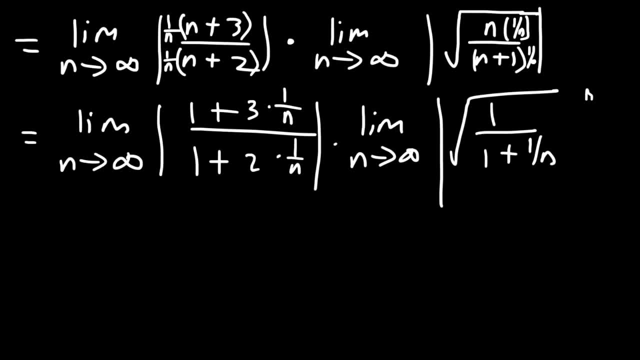 1 over n, all within the square root symbol. So as n goes to infinity, 1 over n becomes 0. So we're going to have 1 plus 3 times 0 over 1 plus 2 times 0.. 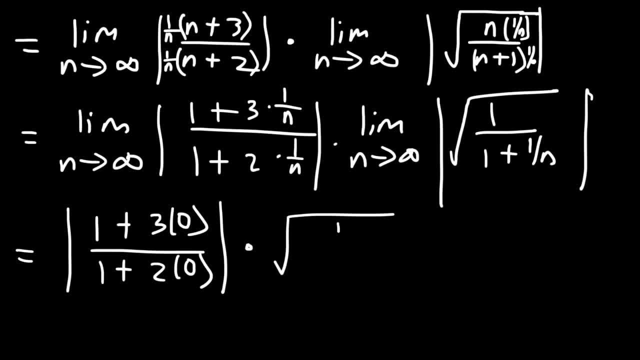 And then for this one it's just going to be the square root of 1 over 1 plus 0. So 3 times 0 and 2 times 0, that's just 1.. So we have 1 over 1, and then times the square root of 1.. 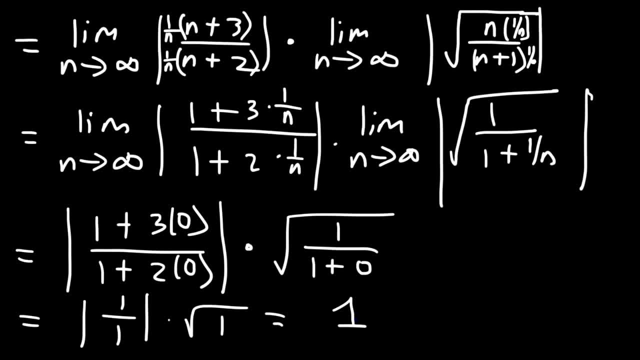 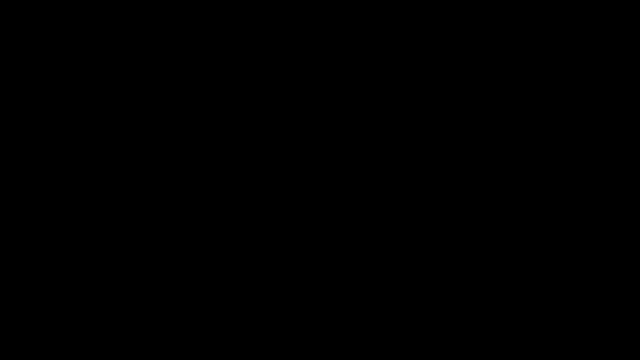 So the whole thing is equal to 1,, which means that the series is inconclusive. We don't know if it's going to converge and we don't know if it's going to diverge. Thank you.